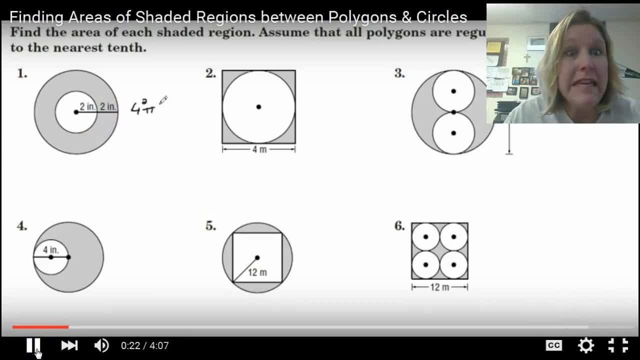 Now we need to be able to subtract the inside circle. The inside circle would be a 2 as a radius, so 2 squared times pi. Now, as you do that, if you were estimating you would say 4 times 4 is 16.. 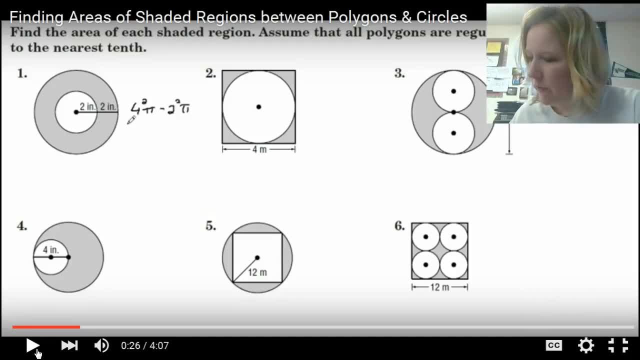 16 times 3.14 would be 50.24 if you're going to be exact. That's not necessarily the estimate, but let's see Then the smaller one, if you do 4 times pi, because 2 times 2 or 2 squared would be 4,. 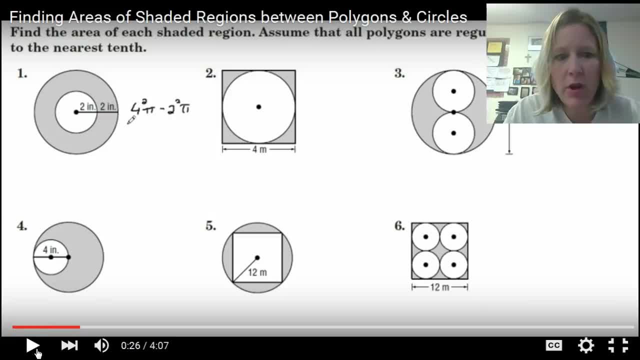 times pi is 12, and we're going to subtract that 12 from our 50, and let's see how close that gets us. So the 12 is going to be Subtracted from: Oh, we wrote 4, and we should have wrote from the 50, and it became about 7.7.. 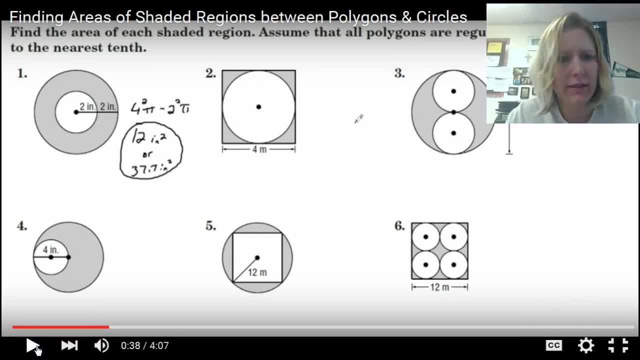 I got 37.68, not 37.7.. On a test you're going to be around that. So you normally are able to eliminate answers that aren't reasonable just by even doing estimation. So you know you're going to be close to around 40, and your answer should be there. 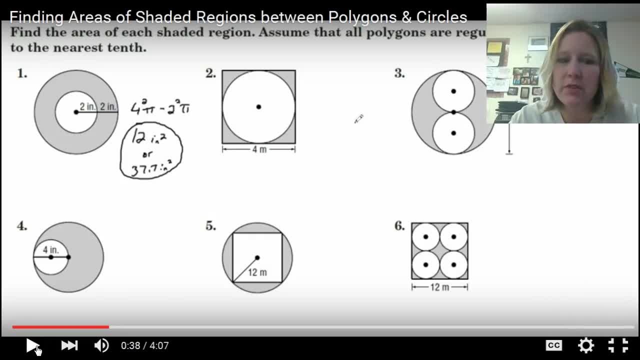 But let's start using 3.14 when you see those 3.14.. 3.14.. We're going to use decimals to make sure we're being more exact. All right, let's move on to the next one here. 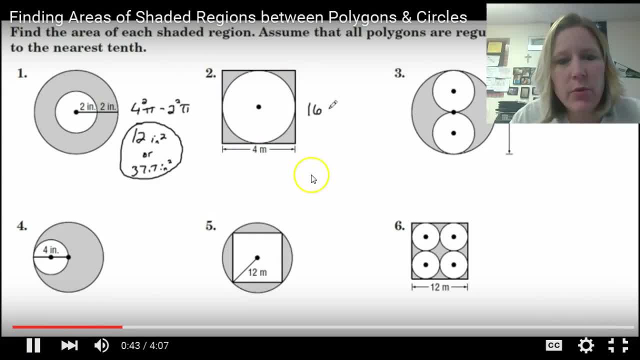 This time we're dealing with a square, So we know that this way is 4, which this way would be 4.. That's going to be an area of 16 for the square, and then we're going to subtract the inside radius. 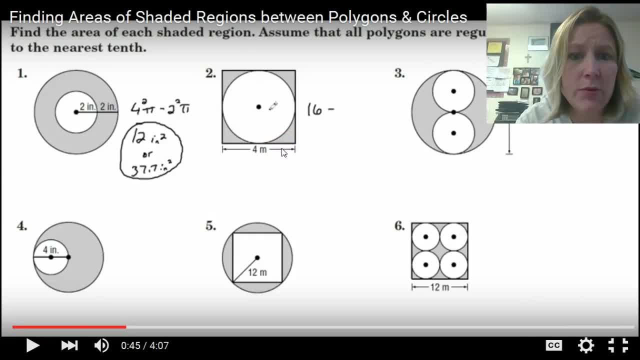 Oh no, The radius isn't labeled. What do you think that radius would be? Well, it's got 4 for the whole thing, so halfway will be 2.. So we're going to have a radius of 2.. Let's keep this going. 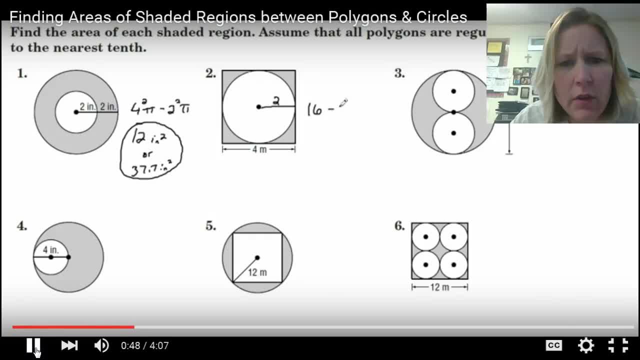 2 squared Times pi to find the area on this one. So that's just like the last one. We had 50 point. 50 point, He's too fast for me. No, Radius times radius. Oh, we already did the radius times radius. 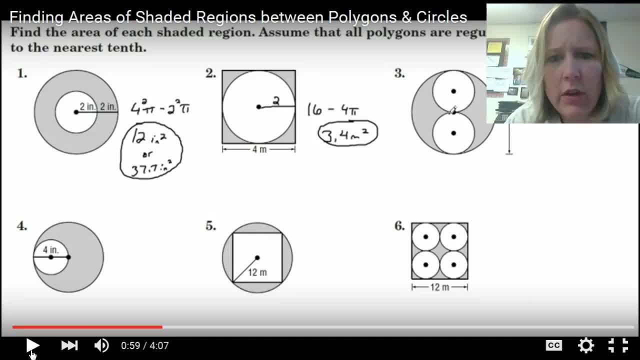 So we actually got 12 as our estimate instead of, Because 4 times pi would be about 12.. So we're estimating there that 16 minus 12. Would be around 3. And we must use the exact here to have it 3.4, because technically pi is 3.14.. 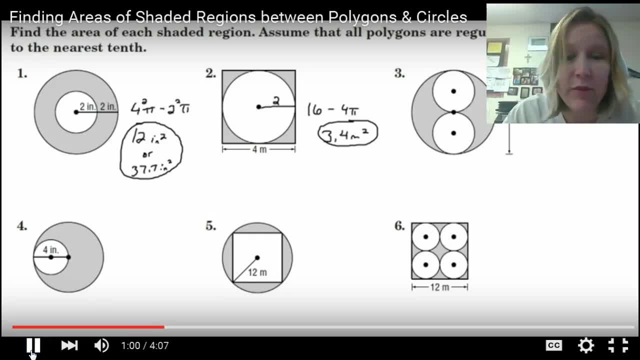 Alright, these examples go fast. I'm going to keep this up, but at least we'll finish the video fast. Alright, the next one. This one is crazy town. Oh, I'm in the way, Let's float me down here. 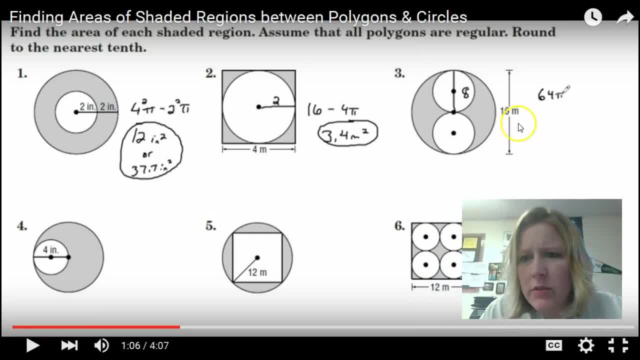 We'll go here instead. Okay, so the radius of this circle is: Oh, because there's two of them. So we went ahead and said We could just pretend. No, I don't understand, Because the radius here The whole thing is 16, so half would be 4.. 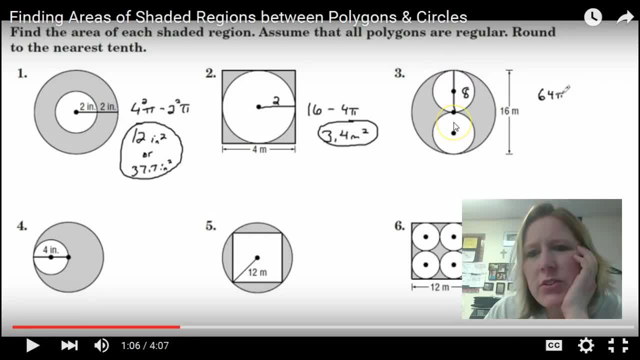 So you would do. Oh, because there's two of them. How'd they get 64?? I may need to actually listen to the audio on this one. Let's see. How'd they get 64?? The circle has a radius of 8.. 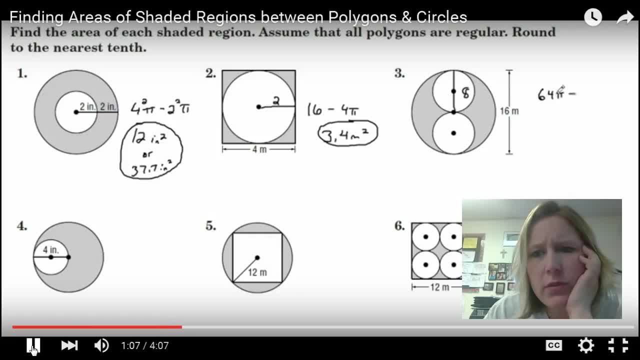 8 squared is 64. So we have 64 pi Minus. Oh, he's doing the big circle, Oh, not the little circles. Okay, it makes sense now. So 64 would be this big circle, Because the radius of the big circle 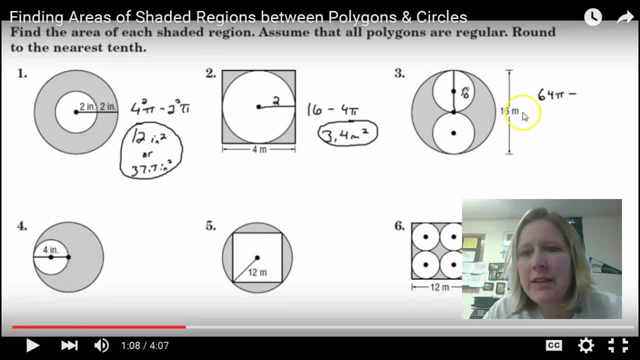 I would have drawn it this way- Is 8.. So 8 times 8 is 64. Pi minus. let's do the inside circles, Two smaller circles, So I have two of them Times pi, And the radius of each of those is 4.. 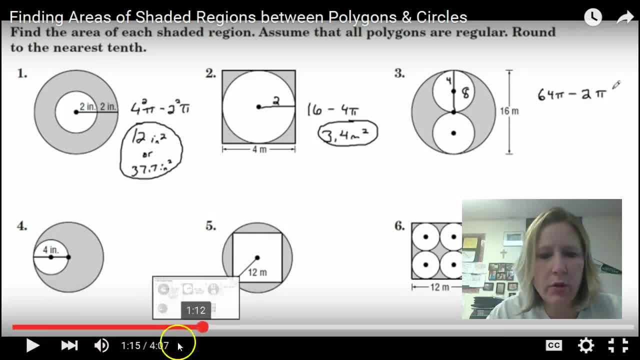 Ah, okay, The radius on those two smaller ones are going to be the 4.. So 4 times 4 is 16.. So that whole formula is basically saying the big circle minus the two smaller circles, And the two smaller circles have a radius of 4.. 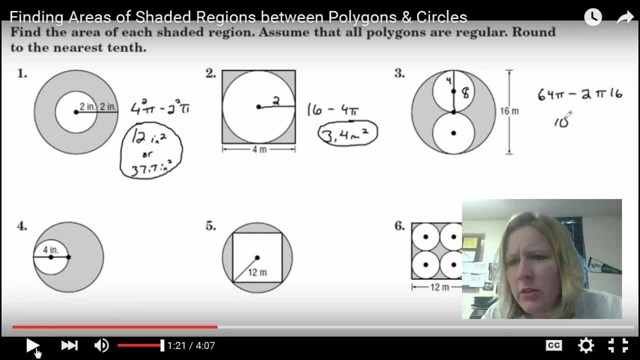 4 squared is 16.. Alright, slowing it down, figuring it out, So that would give us Obviously someone's using a calculator here, Because I would not have done it that quickly. At least we're showing how to set up these formulas. 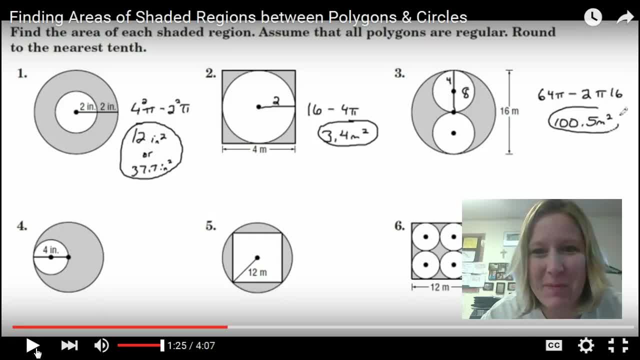 That's a real big part of just figuring out how to set up these formulas and calculate it out. Alright, I bet I can figure out this next one a little quicker. We've got This inner one. here is 4.. Here's the smaller one. 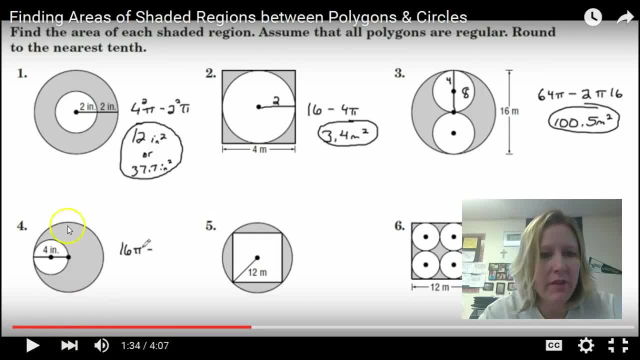 Oh, he's doing the bigger one first. Hello, Let's start with the big one, because we want to figure out the big one, so we know what to subtract. So the big one has a radius of 4.. So that would be 16 times pi. 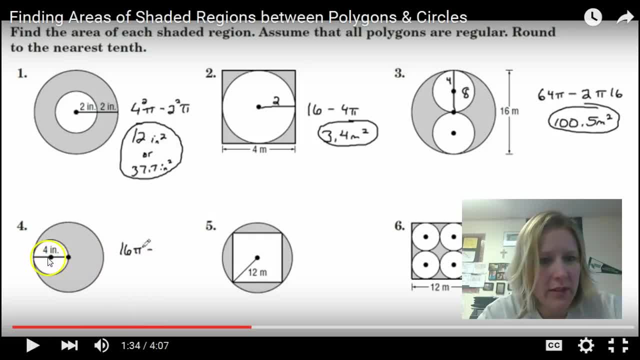 Let's minus. Let's look at the small one. If the whole way is 4, that's the diameter- Then the radius would be 2.. So the radius is 2.. So let's choose 2 to the power of 2. 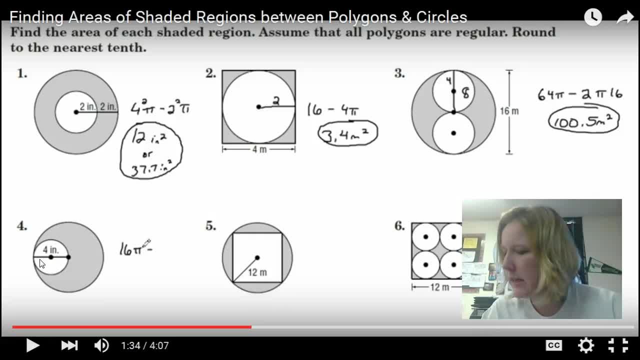 would be 4.. So we're going to take 16 times pi, or 3.14, I'm going to estimate, since he's being exact. So if I do 16 times 3, then I'm going to be subtracting that from 4. 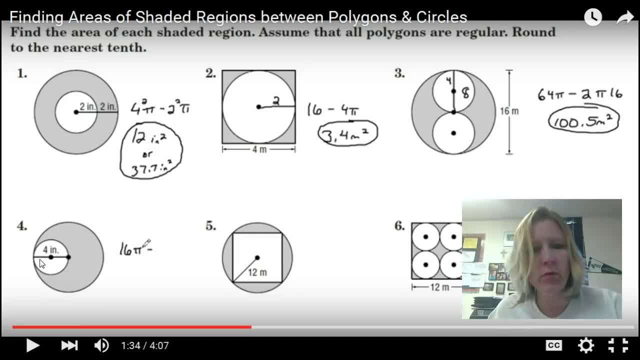 times 3, because radius times, radius 2 times 2 would be 4.. It's going to be about 12.. Let's see if I did that correctly. So we take our 16, so the smaller radius is 2.. 2 times 2 is 4.. 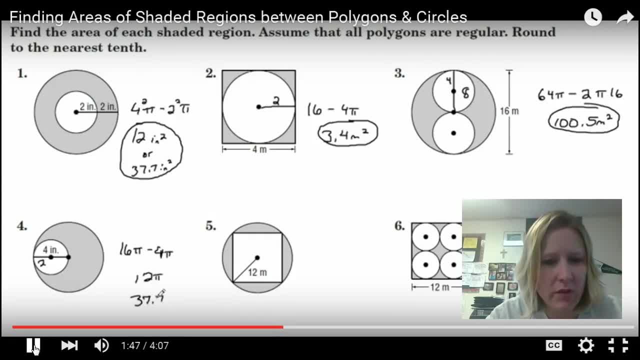 Alright, Then we do get a final answer of about 12.. Why is it saying 37.5 inches? Did I do something wrong? The circle was 16.. 16 squared. Oh, This is just like our first example up top. 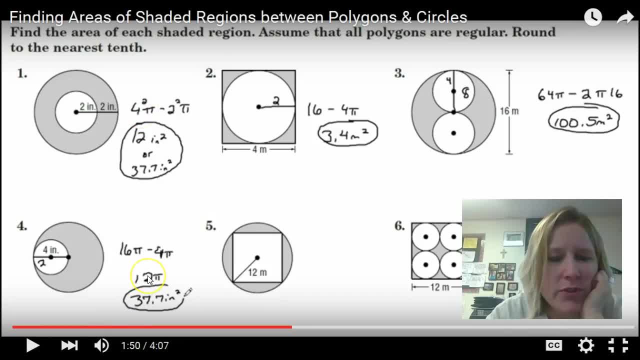 This would have become. 12 is just a smaller one, right? Slow it down. We've got 2 to. the power of 2 is 4.. We're subtracting that out, So you're minusing 12 from the 16 times pi, which would have been 50.. 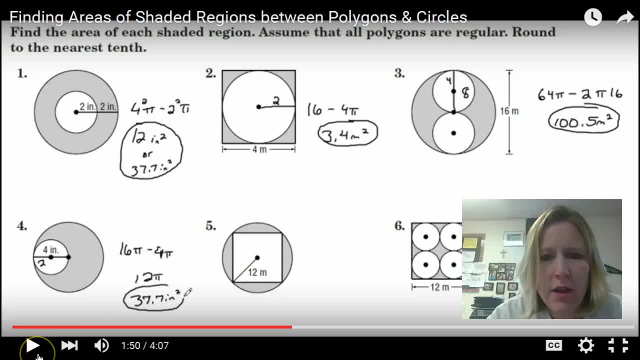 Just like the first one, This one is the exact same answer as number 1.. Alright, I think that's enough examples to kind of get it going. Those next two ones look pretty cool, but I think we're ready to move on. I think this has been enough. 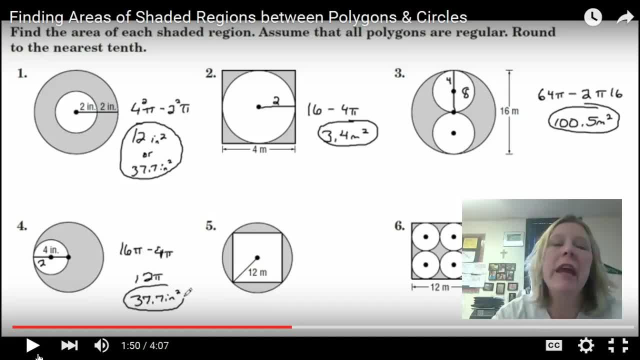 So, thank you, guys so much. Make sure that you're understanding by the end of this, hopefully, how to find the area, that shaded region. If you have questions, let's talk about it during our discussion. Thank you.